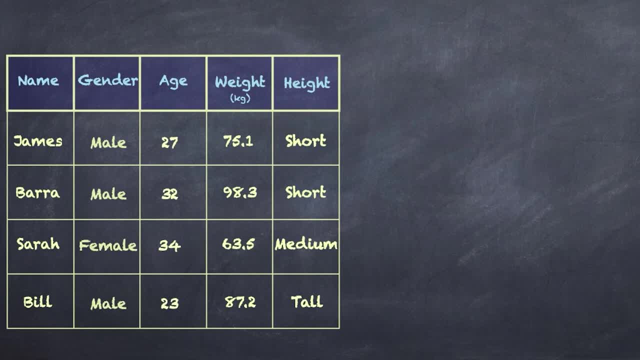 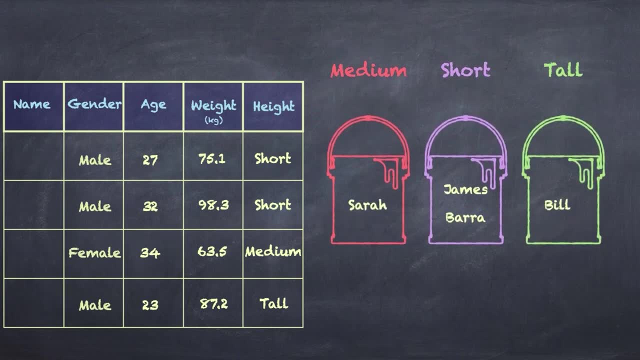 I want to take a look at height. right, And this is what we call an ordinal categorical variable. Now, in the case of height, again we've got categories or buckets, And of course, again we can categorize the observations in our data set. But in this case the order matters, right. 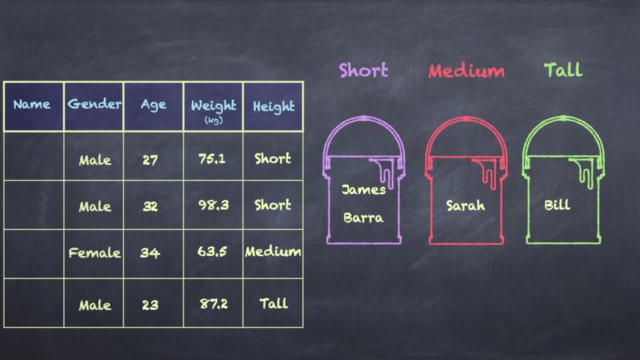 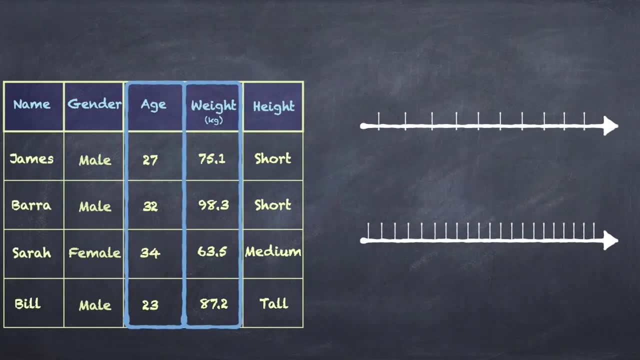 So it's short, medium, tall that matters, And that's why we call it an ordinal categorical variable. There's a natural order to the categories. Now let's talk about the two types of numeric variables. These are numbers. They fall by. 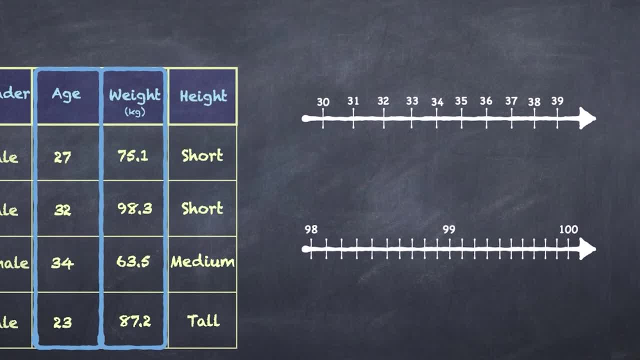 definition on a number line. but they can fall on that number line in two different ways. They can be discrete or continuous. Right, Let's talk about age. Age is typically given as a discrete variable, In other words, each observation falls definitively on a value, on the integer number. 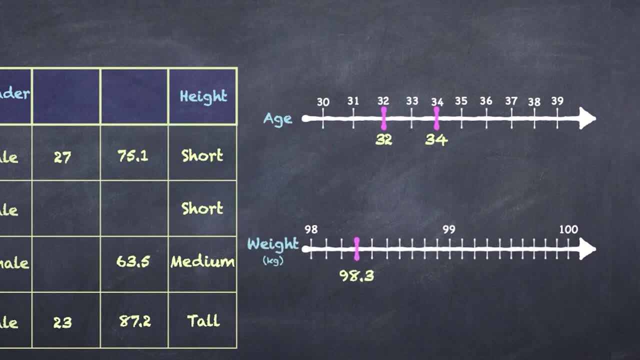 line 32,, 33,, 34, etc. Weight by contrast falls on any number, including fractions between two integers, right? So in this example, Barra is 98.3 kilograms. But now we want to talk about how it. 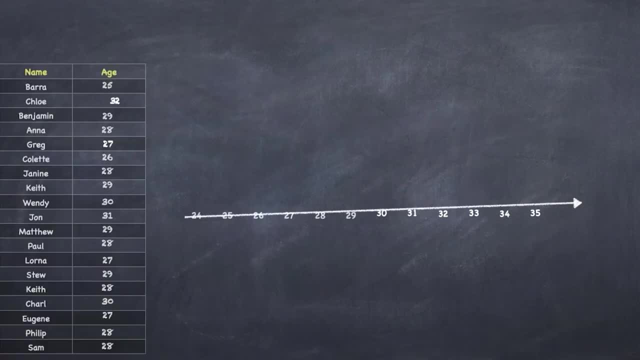 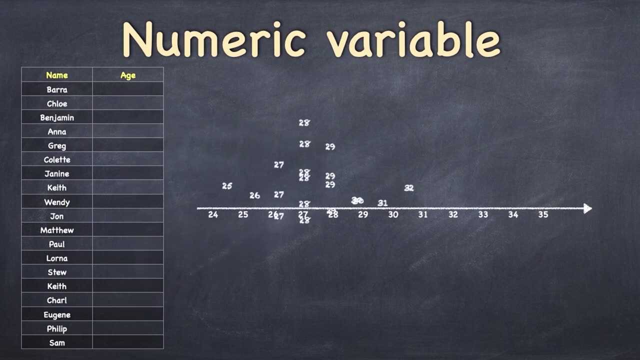 is that we're going to describe all of these variables. A trick to understanding how your numeric variable values are distributed along the number line is to imagine them actually sitting on the number line. Where there is more than one observation for a particular number they get. 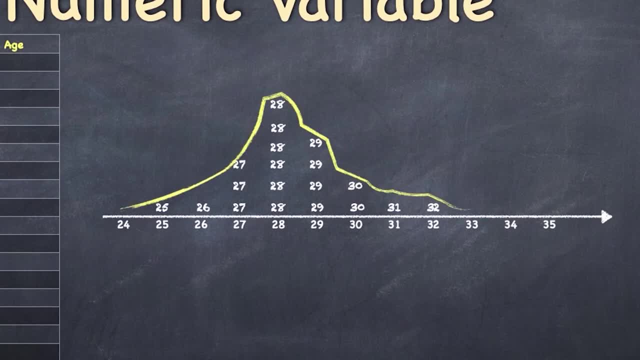 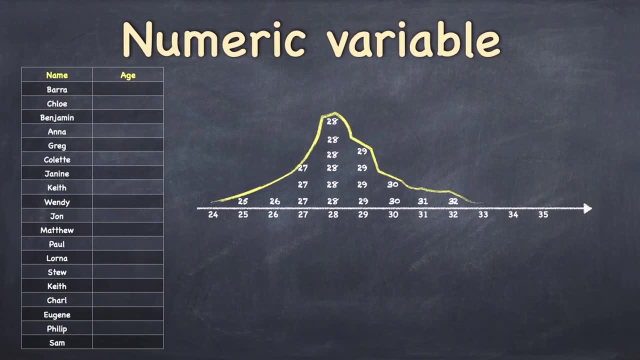 stacked upon each other And, as you can see, this turns into an interesting shape, which we call a distribution, And this is an interesting idea that we use again and again and again in statistics. So here we've got a data set and I've shown the distribution of the numeric variables by. 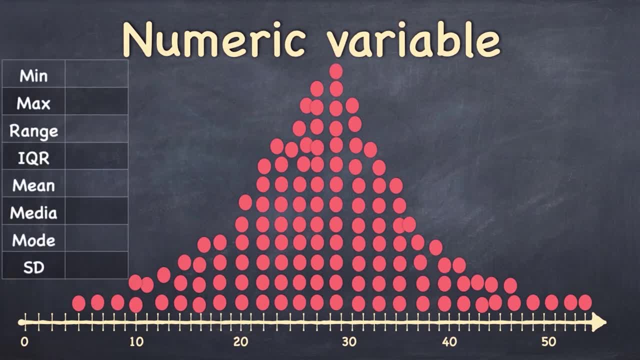 representing each observation as a ball. Let's take a look at the most useful ways that we can describe this data. Firstly, the minimum and the maximum values, And these also happen to be the parameters for the range, And the range tells us a little bit about the distribution or the spread. 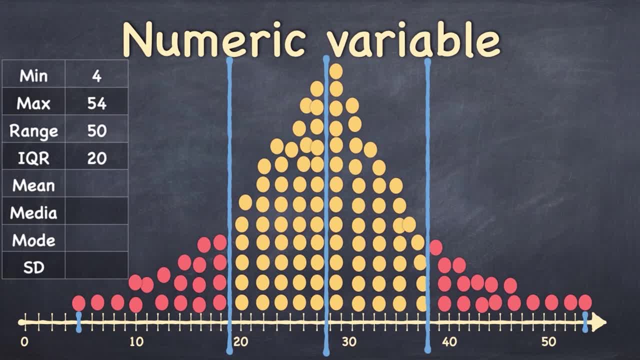 of the data And if we divide all of our observations into four equal groups, each of those groups will of course contain a quarter of all the observations, And we call the two middle quarters the interquartile range, And this again is telling us something about how the 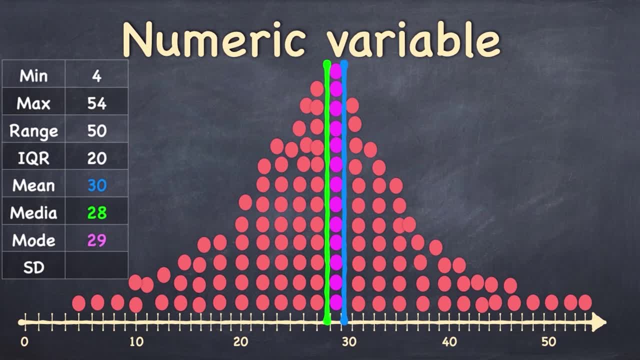 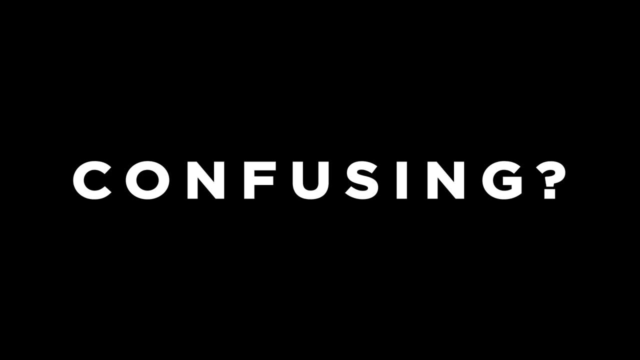 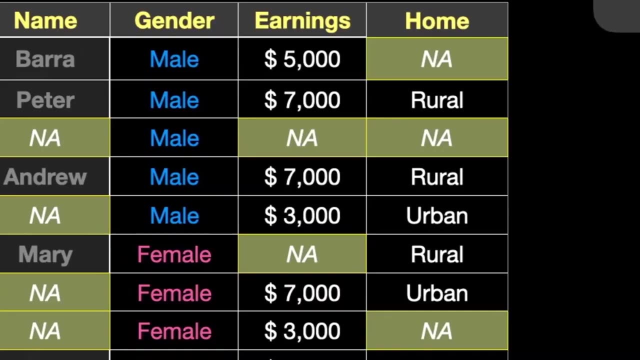 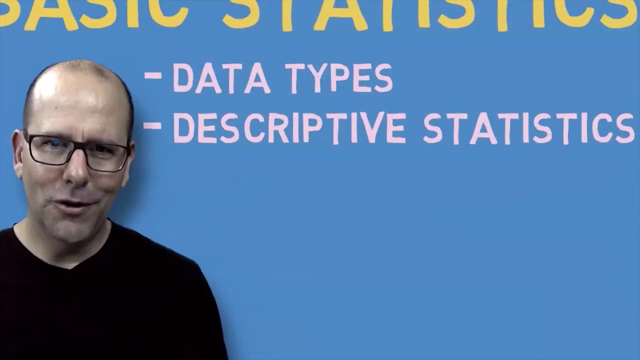 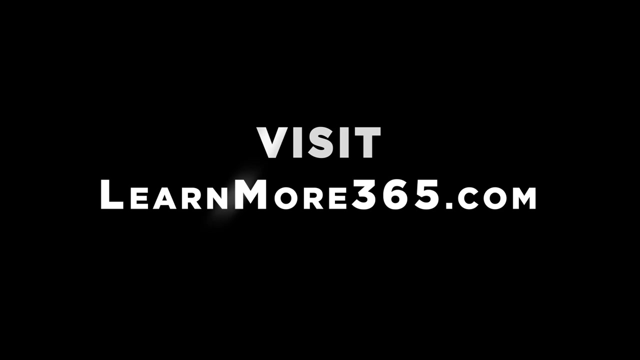 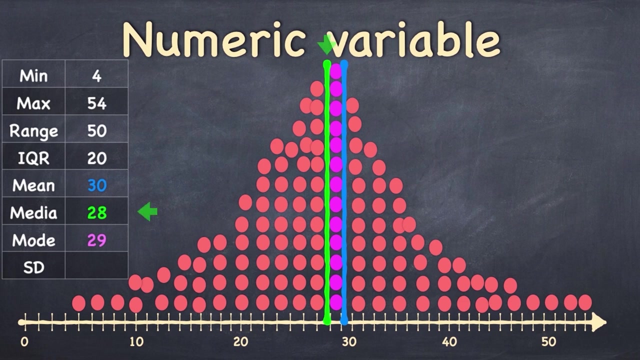 data is spread out. Now. the next three are interesting because they're trying to tell us something about the middle of the data. Welcome to the course on basic statistics. So sit back, enjoy, buckle up. Let's do this. First of all, we've got the mean. The mean is the average. Then we've got the median And the 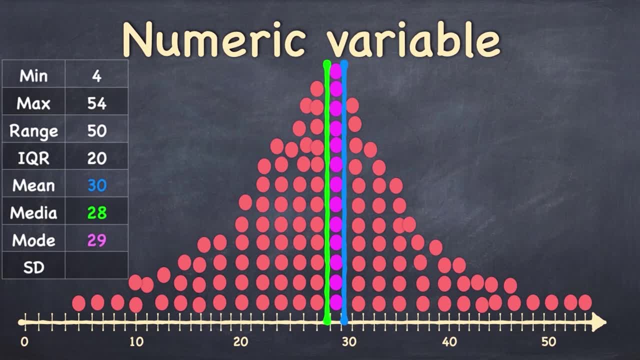 median is the value that splits all of the data into two equal groups. And then, of course, we've got the mode, which is the most common value. Now, where the distribution or the shape of this data is pretty important, we're going to look at the distribution of the data And we're going to look at 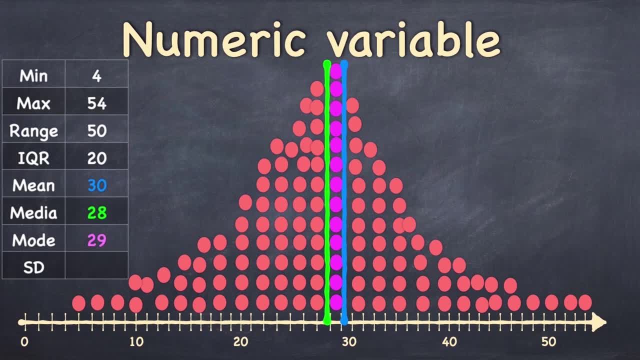 the distribution of the data. Now, the distribution of the data is pretty important. we're going to look at the distribution of the data And we're going to look at the distribution of the data, As in this case, then those three values will be pretty much the same. However, if the distribution 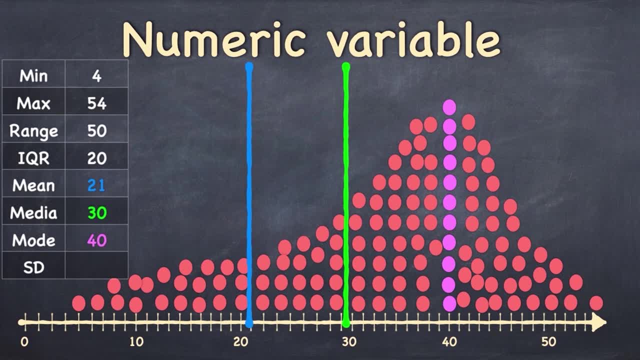 of values has got a long tail to the one side- right, the left side in this case- and we say this is left skewed- then suddenly the mean or the average is disproportionately affected by the outliers and these extreme values. And similarly, if you have a right skewed distribution. 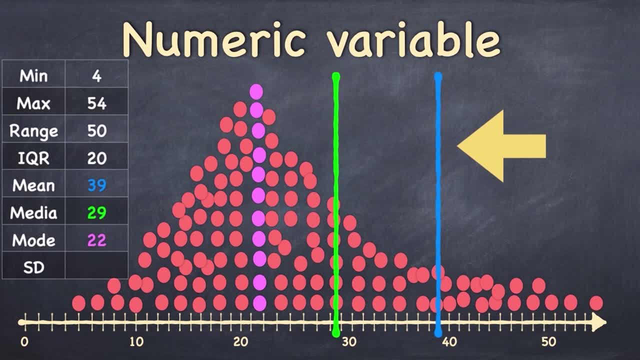 and remember: the tail is to the right, So we say that it's right. skewed the mean is way too far to the right, So it's not a good measure of centralization. And so we've got the two middle quarters And we're going to look at. 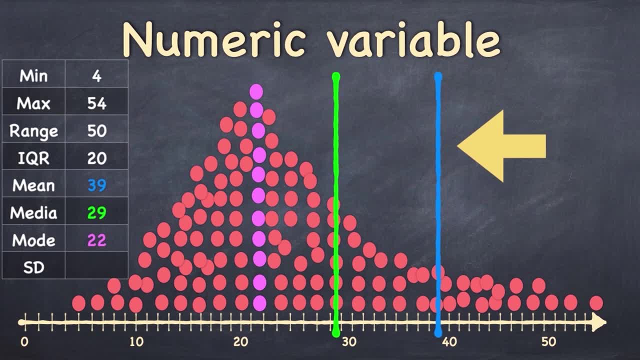 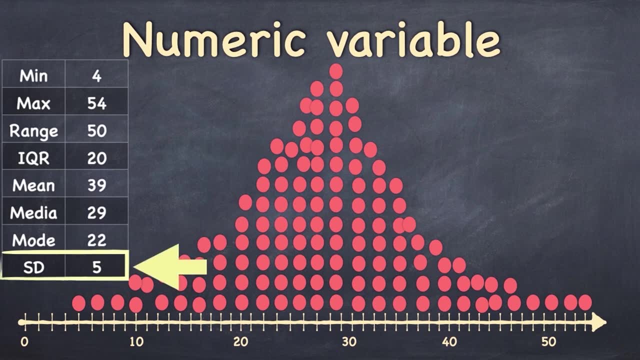 Clearly, when the distribution is skewed, the median is a more robust measure of centrality. And finally, the standard deviation tells us about the average distance from the mean, In other words, how spread out the data is. So if this is the mean, then one standard deviation on either side of that is the average distance of the observations from the mean. 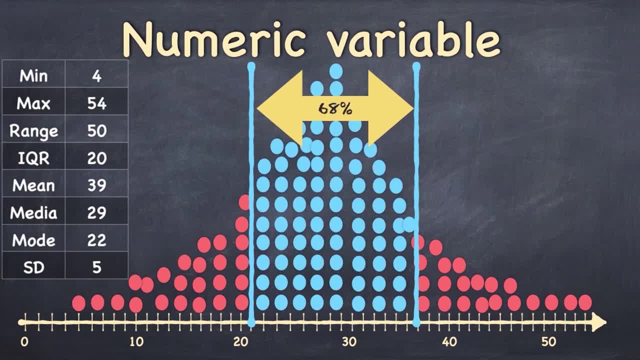 And it turns out that if your data is normally distributed like this is, then about 68% of all of the observations will occur within one standard deviation on either side of the mean And about 95% will be within two standard deviations. So what have we got? We've got the mean, the median and the mode. 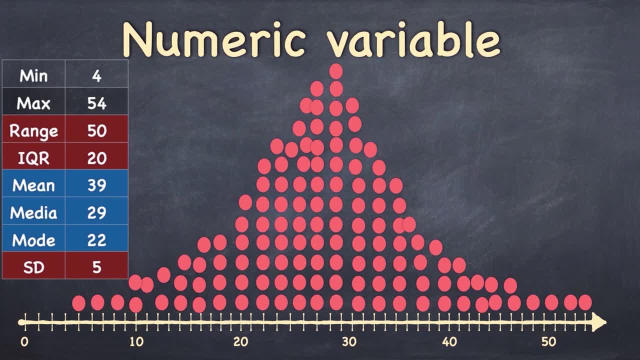 They're telling us about centrality, about the middle- Where's the middle of this data? And then we've got the range, the interquartile range and the standard deviation. And they're telling us about the spread and how spread out this data is. 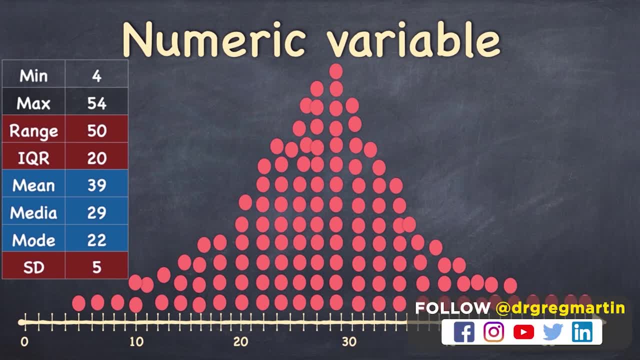 Now we've got terminology. We've also got terminology that tells us about the shape of the distribution. We've already talked about the idea of the distribution being symmetrical or skewed to the left or the right. If there's one peak, like in this particular data, we might say that this is unimodal. 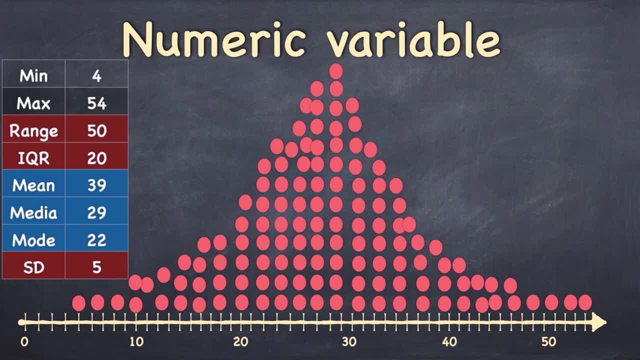 If there were two peaks, we might say that it's bimodal, And there are other distributions that we can talk about. But the best way to get a sense of how to describe the shape of the distribution is to visualize the data. So let's get into that for a bit. 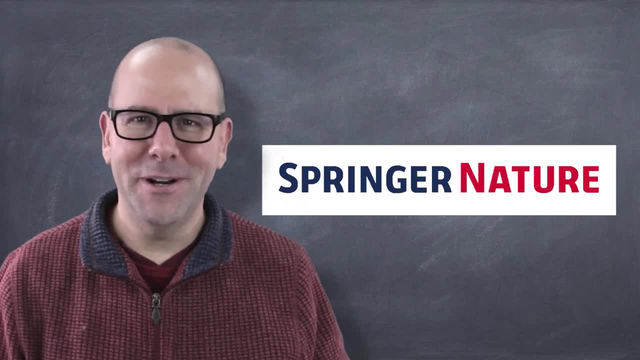 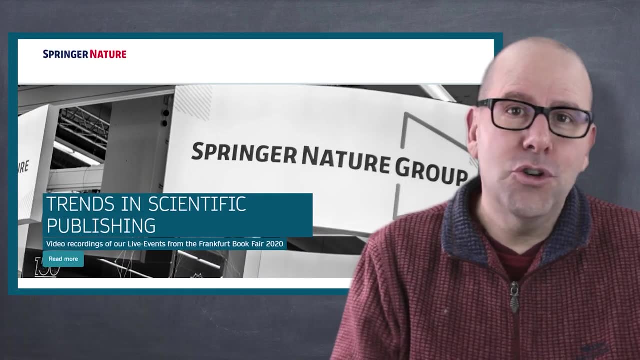 A short pause to this video to say a big thank you to Springer Nature. Now, this video has been sponsored by Springer Nature. Springer Nature did not create the video. They had no editorial involvement with the video. They take no responsibility for the video. 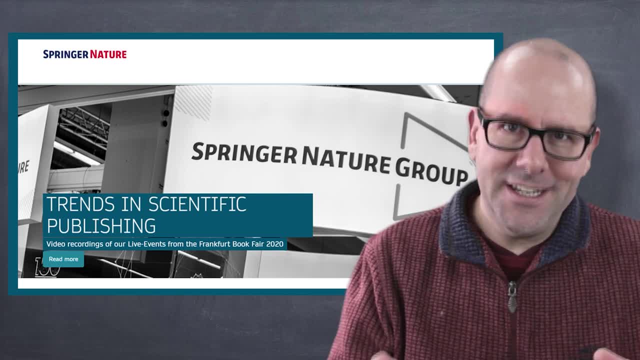 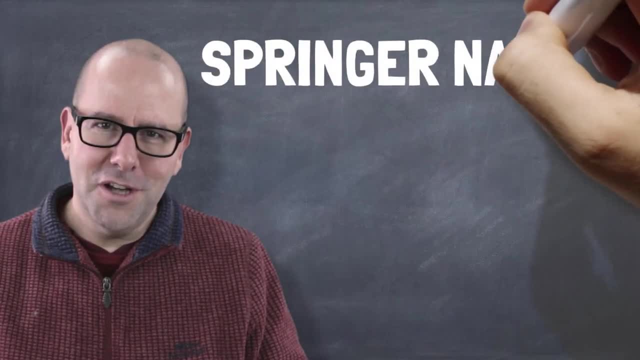 That's the stuff that I'm obliged to contractually say to you. There's a few things about Springer Nature that I want to say to you, that I don't have to say, but I want to say anyway. Springer Nature publish some of the most influential scientific journals in the world today. 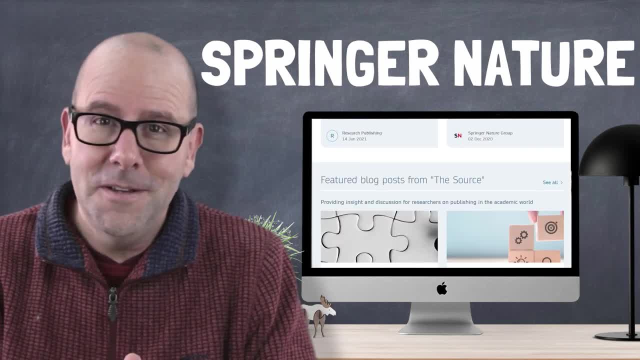 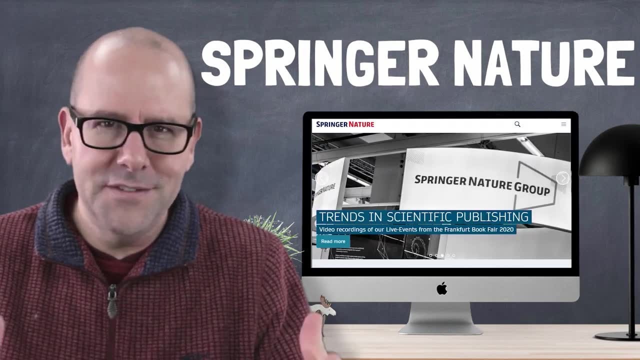 Something that we're not cognizant of in our day-to-day lives is that the science and technology that underpins the lives that we live in today is the science and technology that underpins the lives that we live in today, At the moment, so much of the lives that we live, the medicines that we take, the fact that things work the way they do. 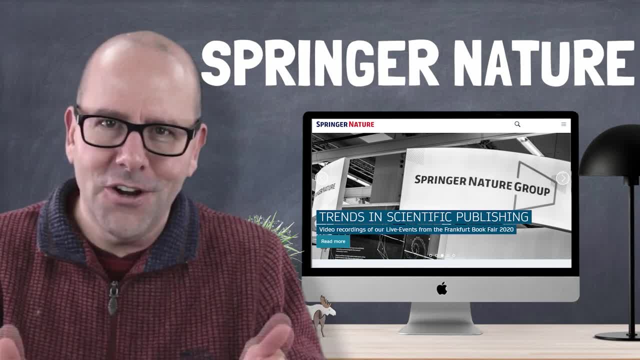 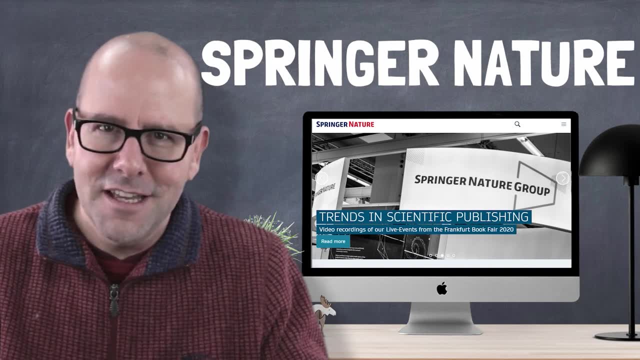 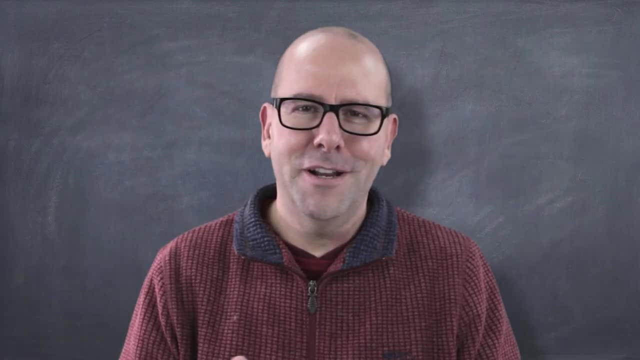 so much of the quality of science that we depend on is underpinned by high-quality scientific publication. It's only of the quality that it is because of publishing companies like Springer Nature that insist on scientific integrity in terms of what they publish. Springer Nature are a real force for good in this world. 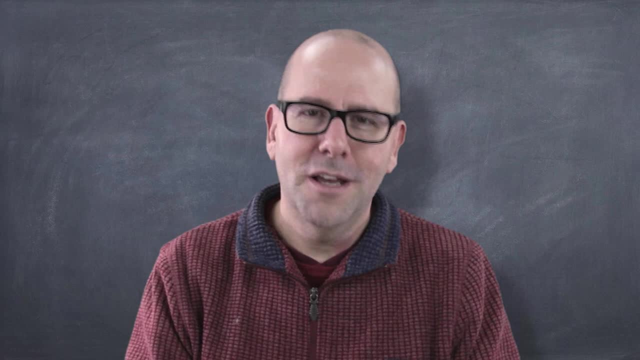 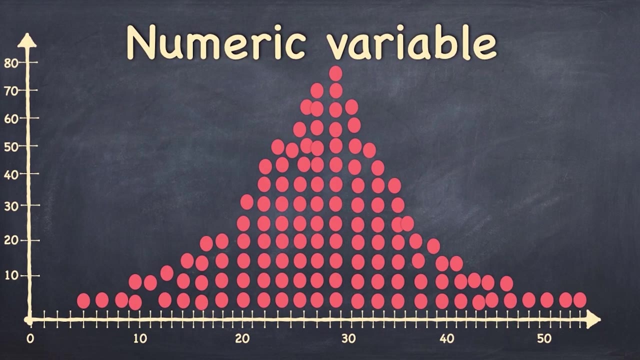 And I feel I'm really grateful and really honored that they're prepared to support my work and this YouTube channel. so thank you very much. And now on with the video. Now, the first way that we can visualize the distribution of a numeric data set is by imagining buckets that represent different intervals along the x-axis. 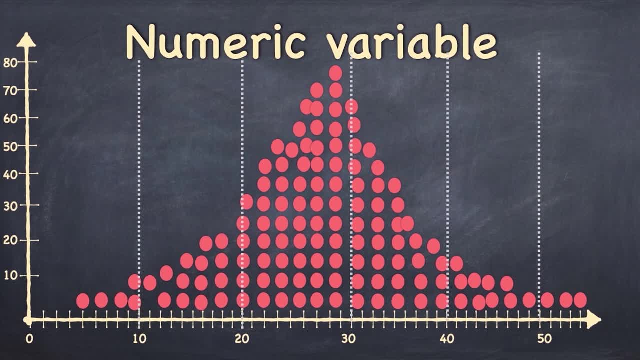 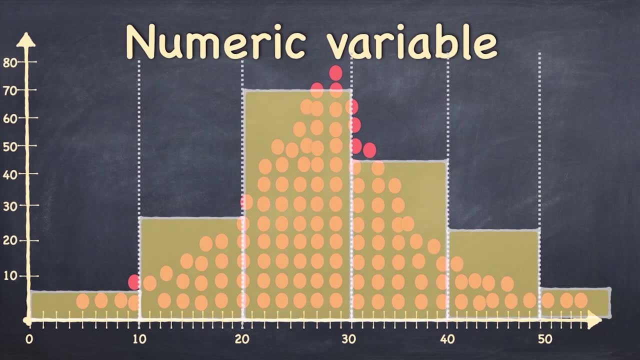 And you can choose how big the buckets are. Let's say, in this case we're going from 0 to 10, 10 to 20,, 20 to 30, etc. And then by counting up how many observations fall into each of those buckets, we can create what we call a histogram. 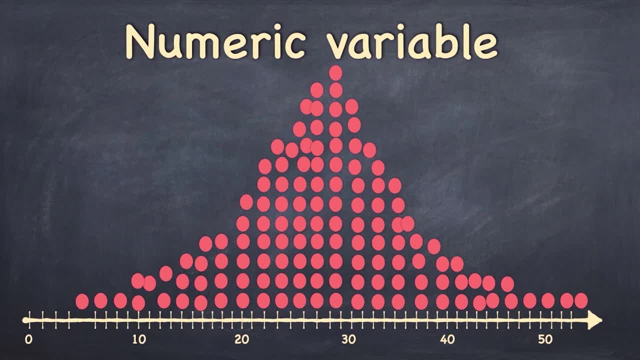 Next, let's talk about box plots, right? Remember when we were describing our data. we divided our data into four quarters, right, And the middle two quarters were described as the interquartile range. Well, we can draw a box that represents the interquartile range, with a line in the middle representing the median. 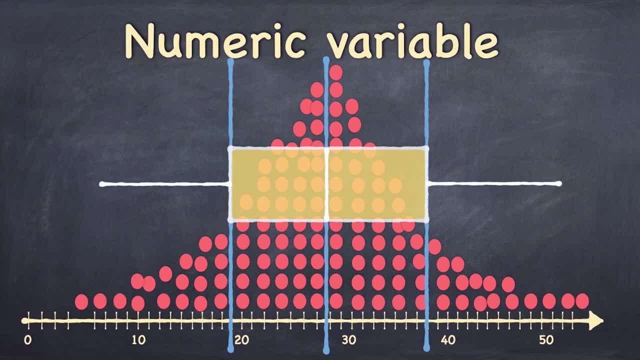 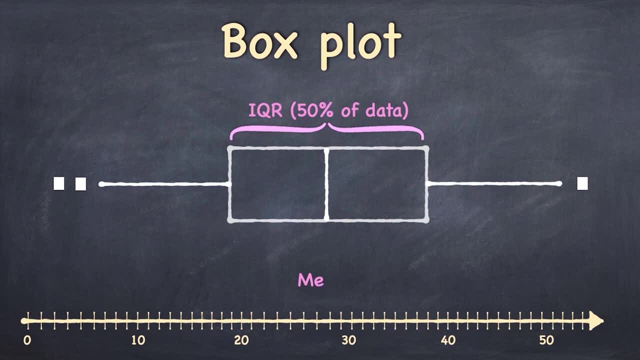 So voila, and we've got a box plot. So with our box plot, the interquartile range is in the box itself and that'll have 50% of the data, The median, which is the value that splits all of the data into two separate groups. 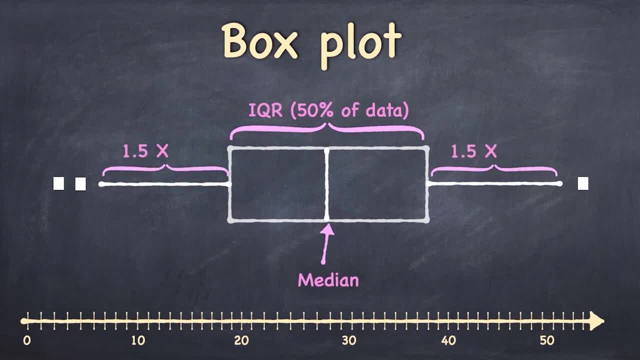 that's represented by the middle line in the middle of the box. The whiskers are extended out to 1.5 times the interquartile range And any values outside of that range. we call them outliers. Now let's take a look at a categorical variable like height. 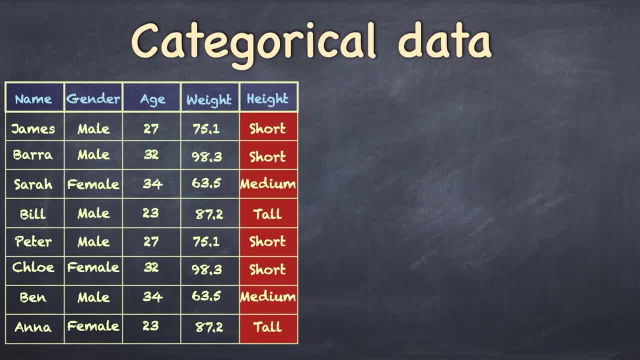 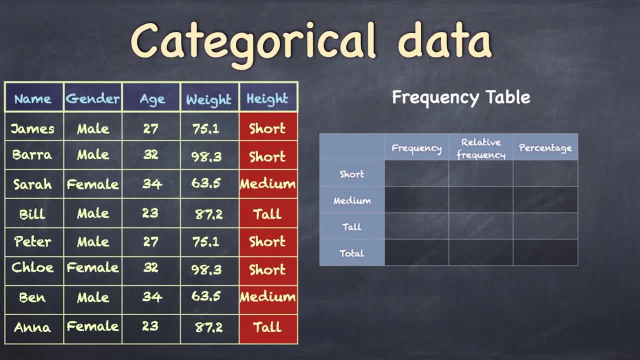 Each observation- so James, Barra, Sarah, etc. etc. has been categorized as either short, medium height or tall right, And we can summarize this categorical variable by counting up the number of observations that land up in each category. 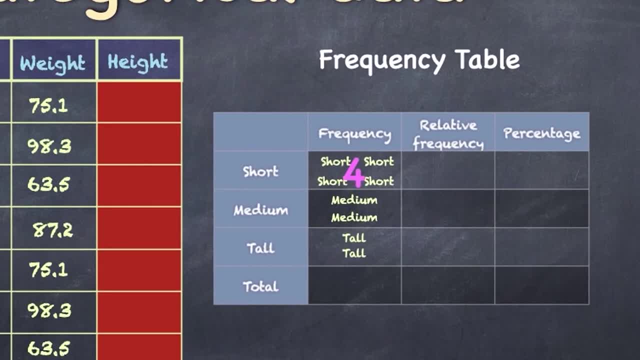 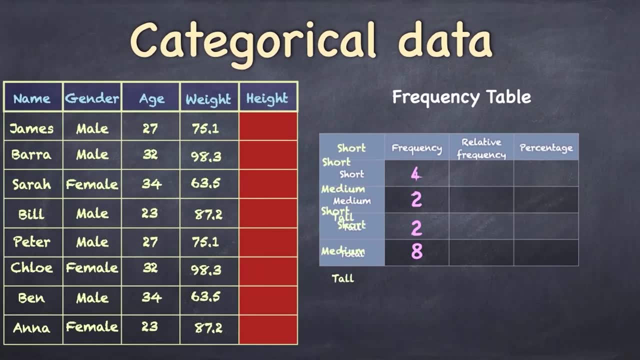 So, for example, we could say that there have been four people that have been categorized as short. We can say that there are two that are medium height, two that are tall and altogether we know that there are eight altogether. Now, if you want to know what proportion of the total are short, right, we call that the relative frequency. 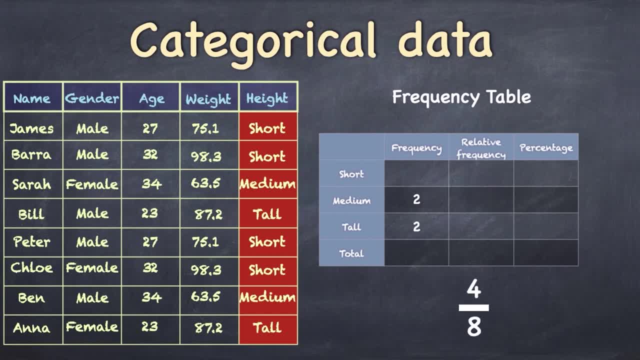 Then, of course, what you do is you divide the number of short people by the total and, boom shakalaka, you've got 0.5, which is a half. And if you want to know what the percentage is, well, you simply multiply by 100. 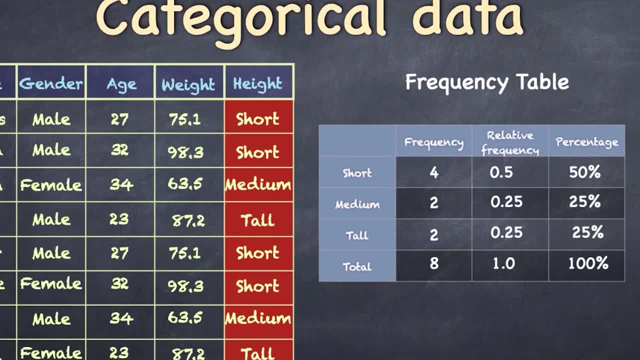 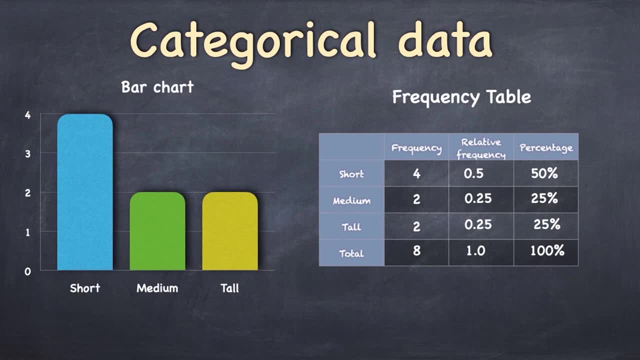 And boom, And there you go. We've got the percentage for each category. If we want to visualize this data, of course we can use a bar chart, where the height of the bar is either the actual number of observations, or the relative frequency, or the percentage. 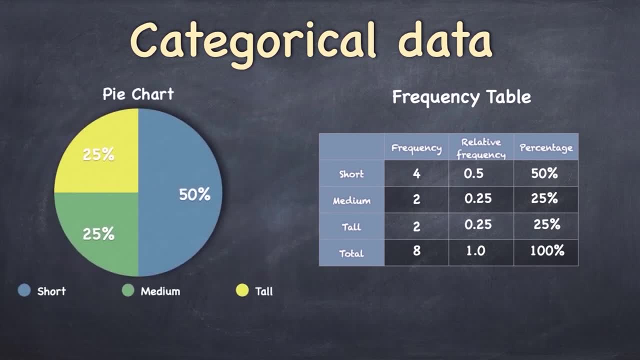 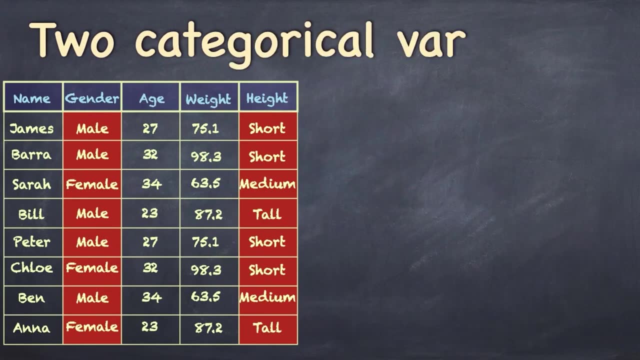 An alternative is to use the pie chart. There are different reasons for using different graphs at different times. I'm not going to get into that today. Now let's think about two categorical variables: right, gender and height. The first thing we do is we create a two-way frequency table. 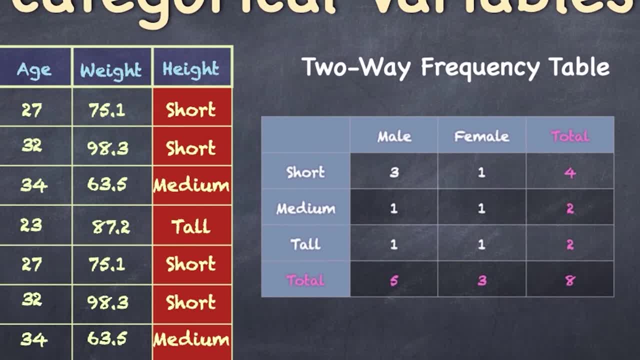 Two ways, because we've got both of our variables involved now and we use one in the columns and one in the rows, And again we can calculate the relative frequency or the percentage which can be represented in brackets next to the value. So previously we had it in a separate column. 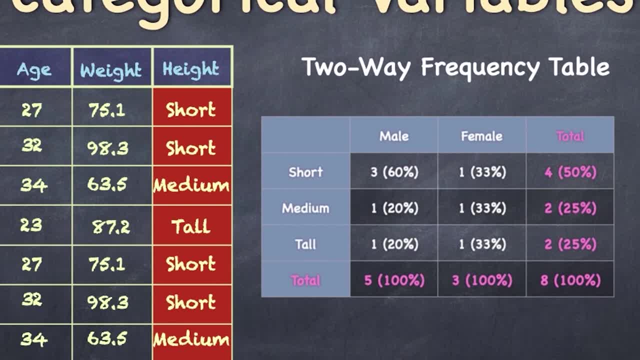 Now we've got it in the brackets next to the value itself And you can do that percentage by rows or by columns, right? So in this case I've done it by columns, So I've calculated what percentage each cell is relative to the column total for the column that it's in. 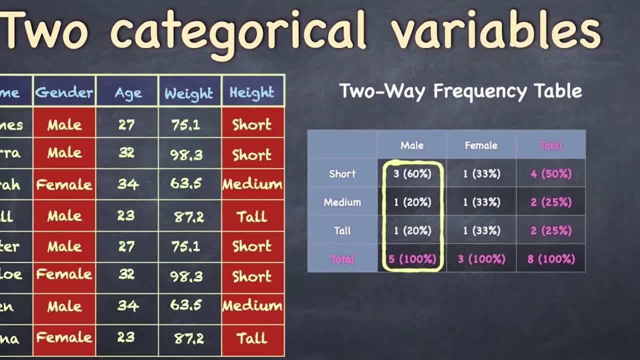 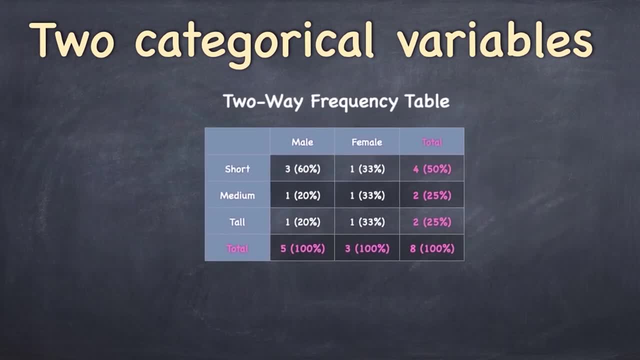 So, for example, in the male column, three men are short. That's three out of a total of five men altogether. So 60% of the men are short, and so on. Now I'm going to show you two ways that you can visualize this data. 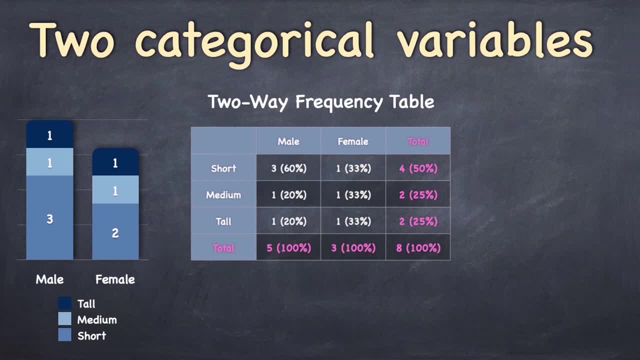 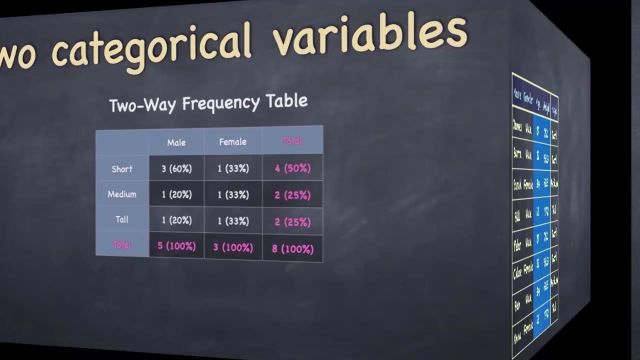 So, firstly, you can have a stacked bar chart where the height of each column is determined by the actual number of observations, Or you can stack them by percentage, so that each column towers up to 100%, making it much easier to visually compare proportions. 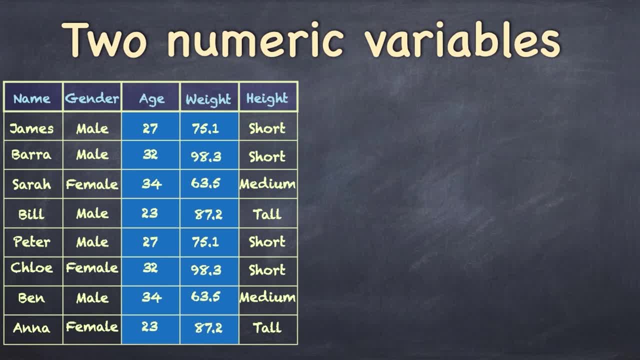 If you have two numeric variables, how are you going to visually represent them? Well, one thing you can do is you can create a scatter plot. So a scatter plot is where each point corresponds to the X and the Y coordinates of a given observation or, in this case, a person. 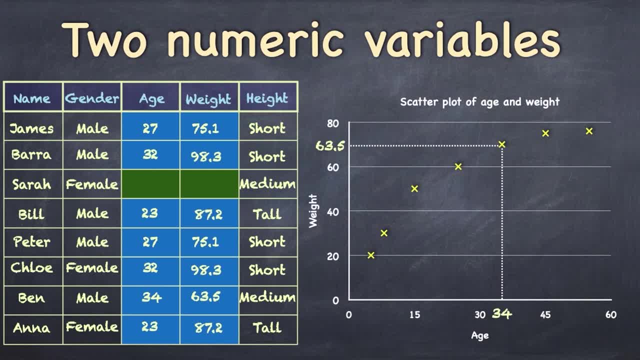 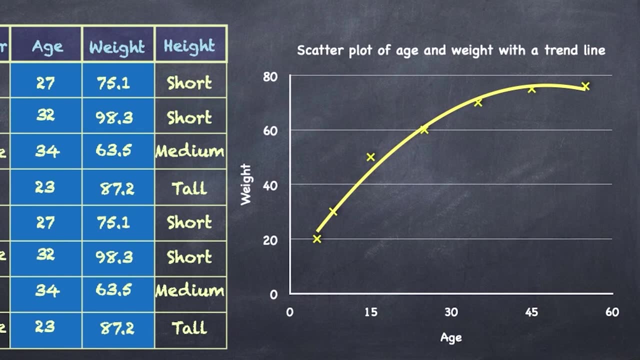 So, for example, we've got Sarah. She's 34 years of age and she weighs 63.5 kilograms. So this is her point on the scatter plot. And of course you can add a trend line. And remember, by convention we usually plot the independent variable on the X axis and the dependent variable on the Y axis. 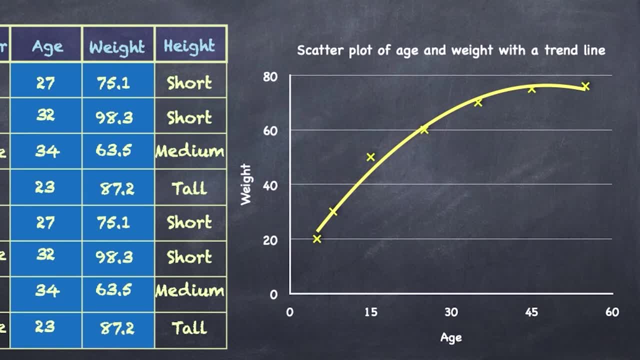 And what do I mean by that? Let me just explain that to you, because it's kind of quite important. It's all about the direction of causation, And so what do I mean by that? In this case, we think that a change in age might affect weight. 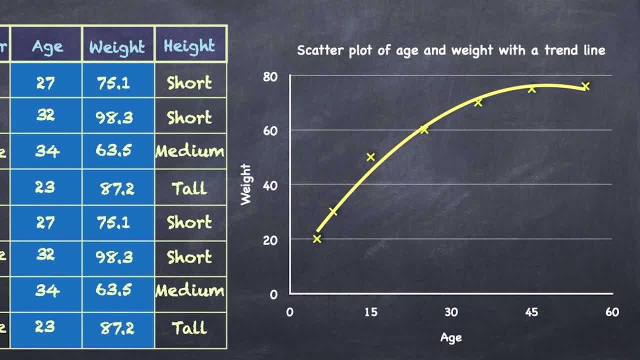 In other words, as you get older, you might gain weight. We don't think that a change in your weight affects or has any causative impact on your age. Weight, by contrast, might be dependent on age or might be affected by age. 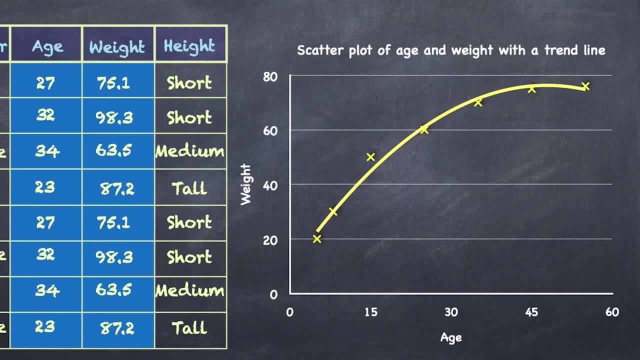 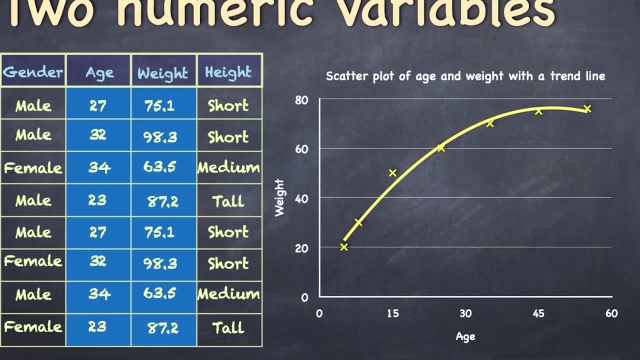 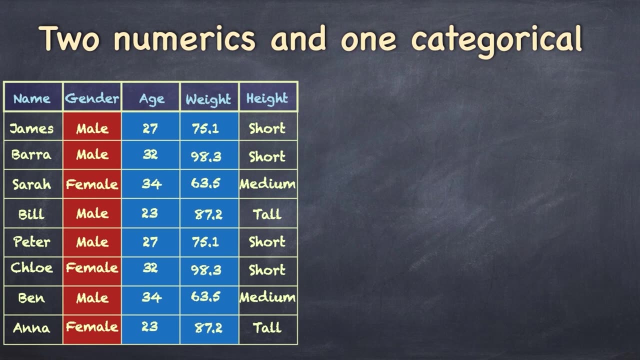 There might be some sort of causative relationship between what your age is and what your weight is, And so weight is a dependent variable. Typically, by convention, we put those onto your Y axis. Now things are about to get interesting. How would we plot two numerics and one categorical variable? 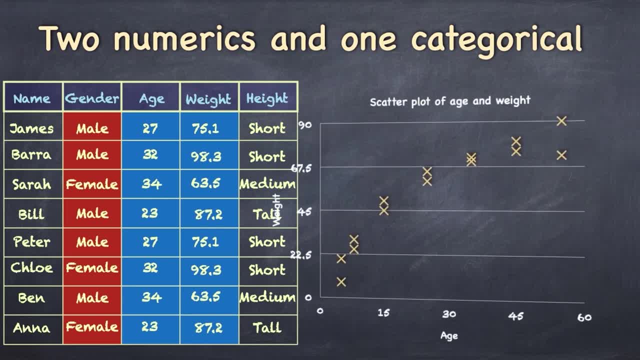 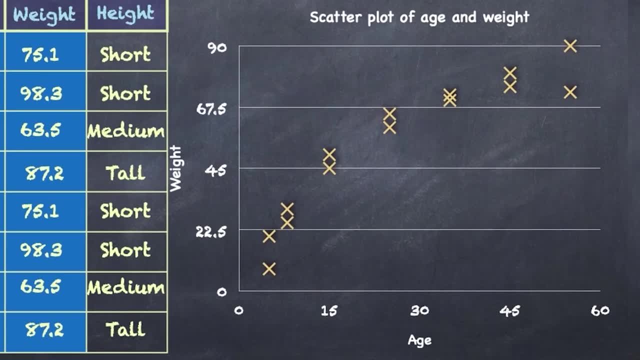 Well, first of all, just imagine plotting your two numeric variables one against each other on a scatter plot in the way that we've described already. Now, for each of the points in the scatter plot, we use the categorical variable to assign them into a different group or a different, in this case maybe a different color. 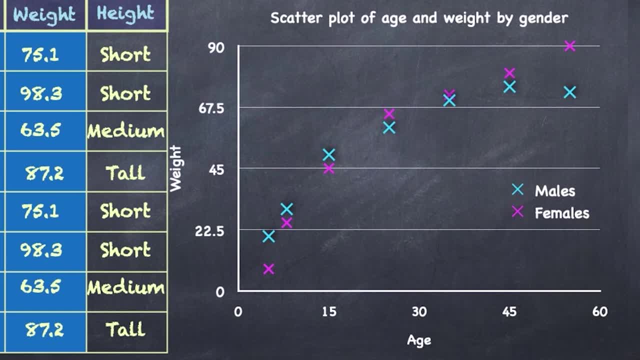 Okay, Then of course we can also draw a trend line independently through each of those points, So we can see the difference between those categories, one for males and one for females. And voila, we can see two graphs superimposed upon one another and we can see the difference between the genders with respect to the relationship between age and weight. 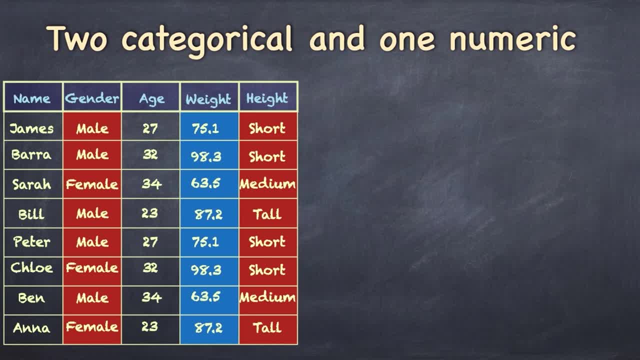 Now let's talk about two categorical and one numeric variable. First of all, let's consider just the numeric variable by itself, in this case weight. And how would we plot that? Well, we'd create, perhaps, a box plot. 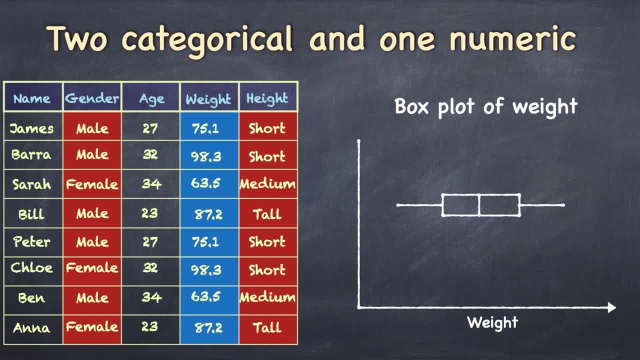 Now we want to use just one of the categorical variables. let's start with gender to disaggregate that data and redraw our box plot. What we've got here is we've got the same weight data being used to draw this plot. Those observations that have been categorized as female have been used to draw the pink plot. 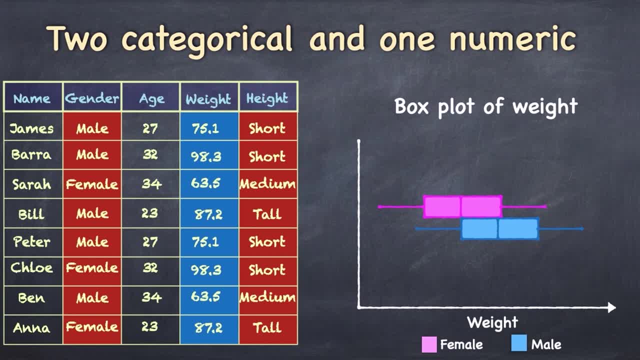 And of course we want to represent more than one categorical variable. We want to include height here. So what do we do? We disaggregate the data once again by height. So now we've got weight and it's plotted, but the plot has been disaggregated by first gender and then height.